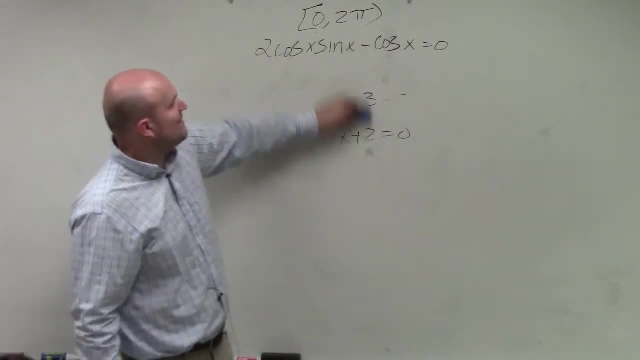 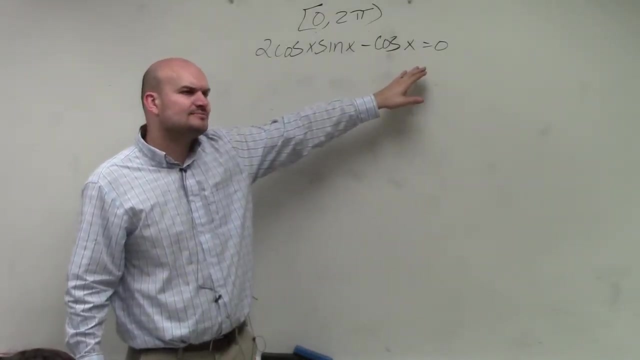 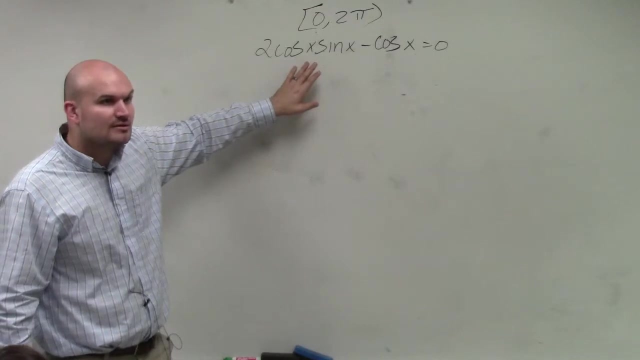 is the case here. You guys can see I have cosine of x and sine of x and cosine of x times sine of x minus cosine of x. I have more than one x. I have more than one x. so I'm not going to be able to isolate just my x, right. So what I'm going to want to do, 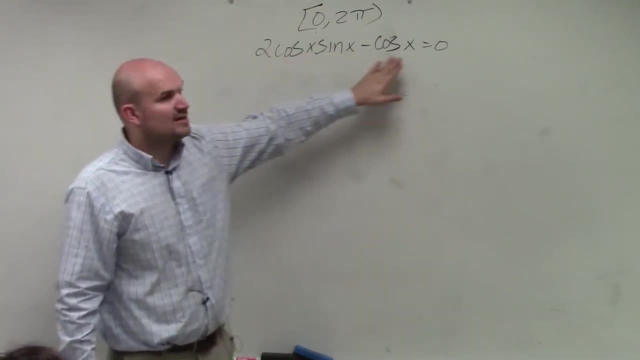 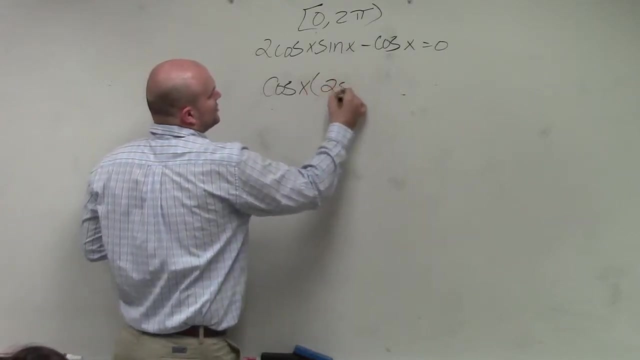 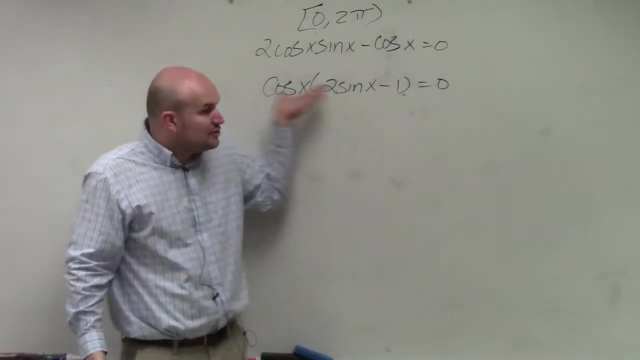 is apply factoring. So is there anything I can factor out of these two terms? Cosine of x. So I factor out a cosine of x and I'm left with 2. sine of x minus 1 equals 0. Now I have the product Zach of two terms set equal to 0. So now I can apply the 0 product. 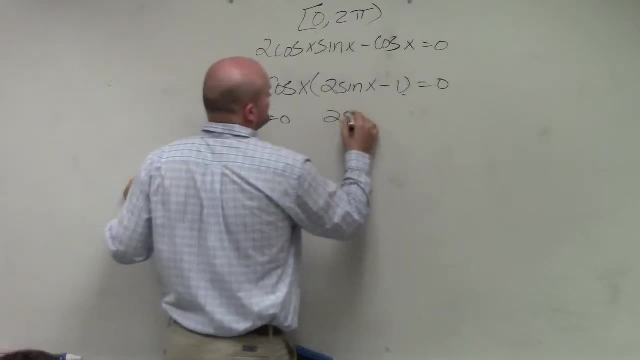 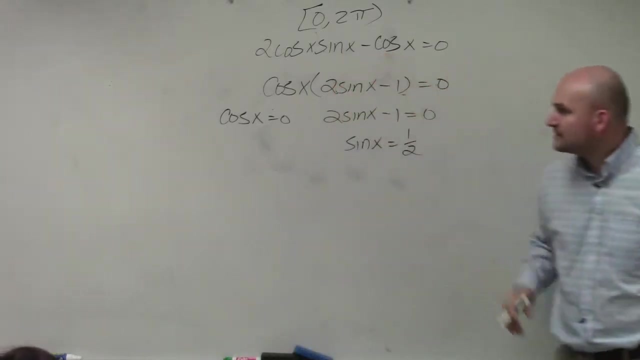 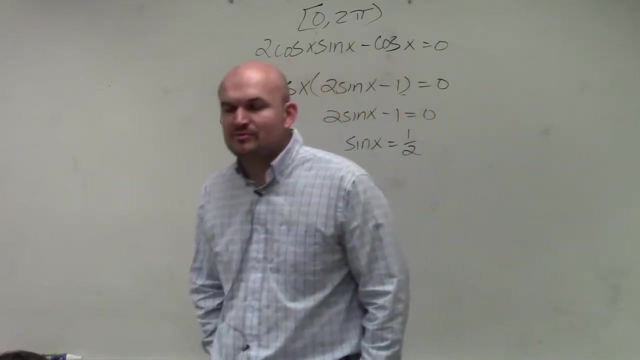 property. So I have cosine of x equals 0, and 2 sine of x minus 1 equals 0, or sine of x equals 1 half. Does everybody follow me Now? if you guys remember, when we were doing these problems, we said the sine of x, or? 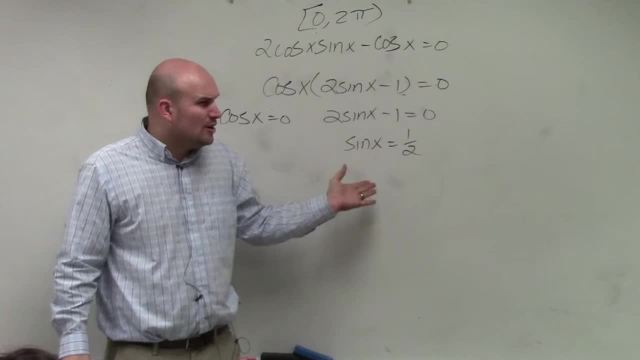 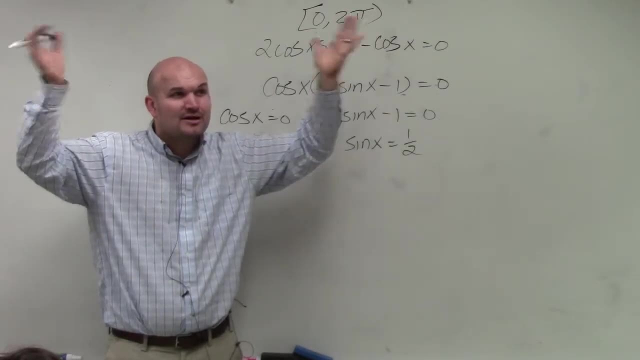 if I said, sine of x equals 1 half. If I asked you for what was x? what does x represent? What am I actually looking for? Is anybody raising their hand? What am I looking for? Yes, it is the answer, but since Sven raised his hand, it's the angle that I'm looking. 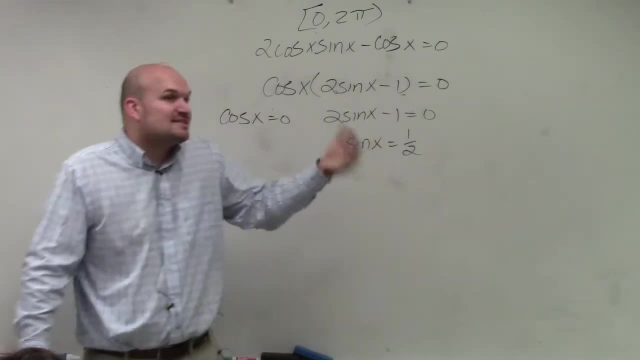 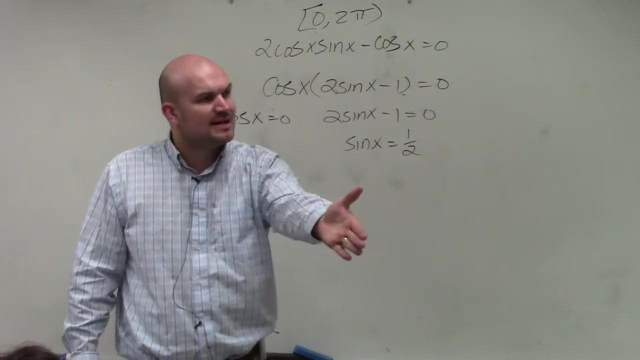 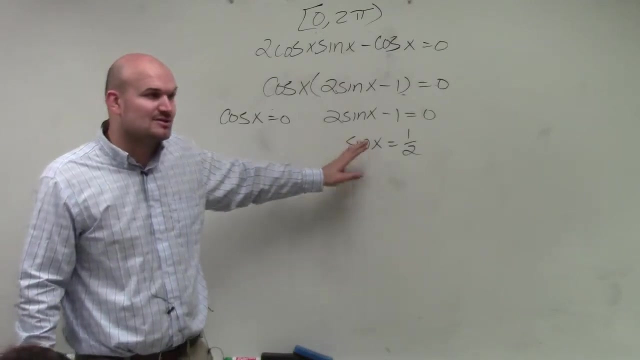 for Sine of what equals 1 half. That means the sine of what angle equals 1 half. correct, The reason why we did our warm up today, the reason why we did that warm up is because now you guys have to know that unit circle and these angles. So what I like to do here, 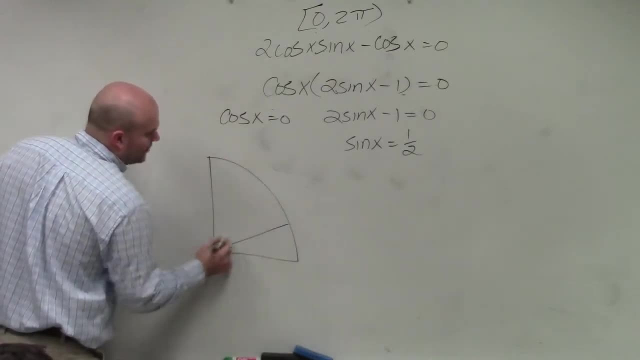 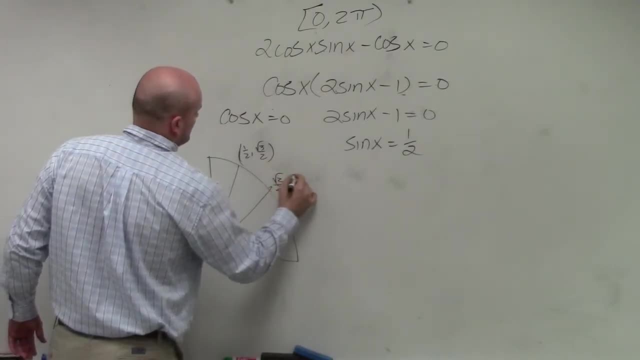 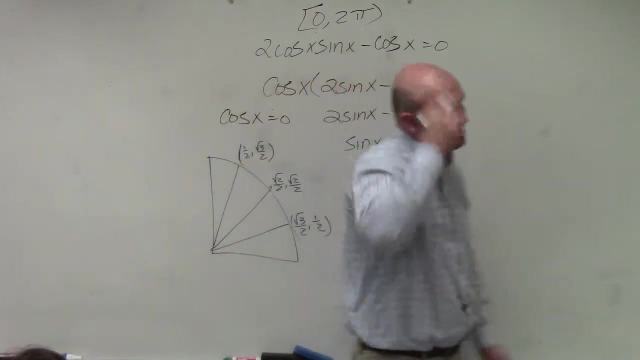 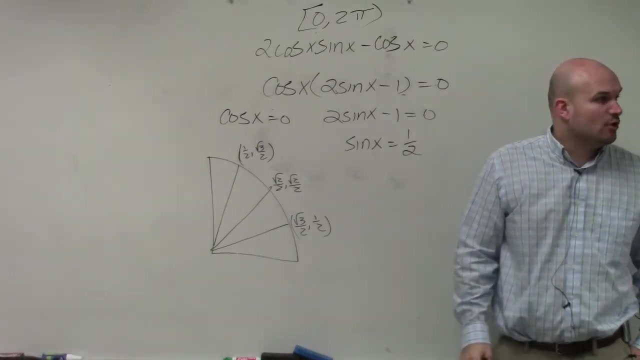 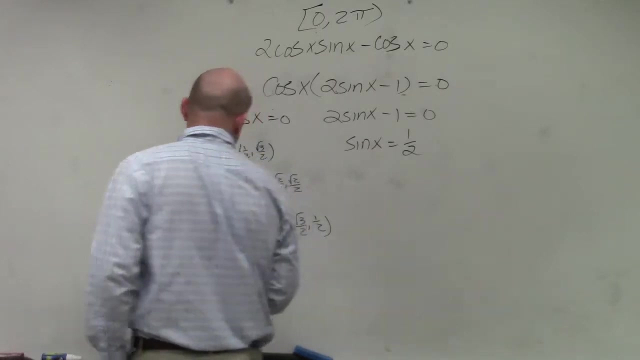 All, right, now all of my answers I'm going to use in radians. So sine equals 1.5, right? So for what angle is the y coordinate equal to 1.5? 30. 30 degrees, but we're going to use our answers as pi over 6.. 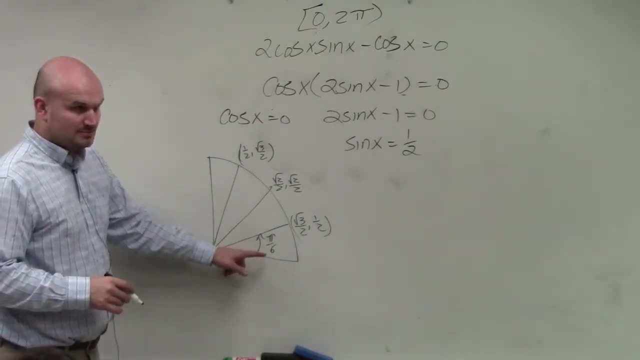 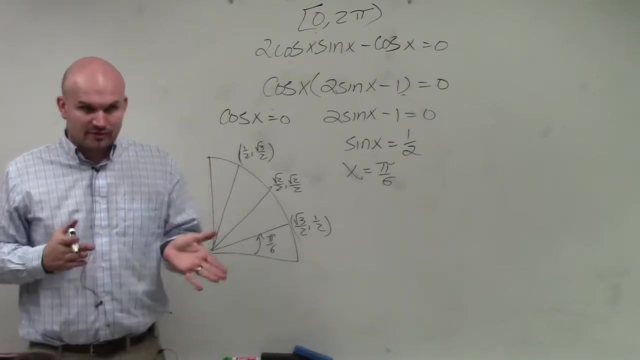 Okay, Does everybody agree with me on that? Okay, So I can say: x equals pi over 6.. However, you have to read the problem very carefully, because what the problem says is: I want you to find all the answers between 0 and 2 pi. 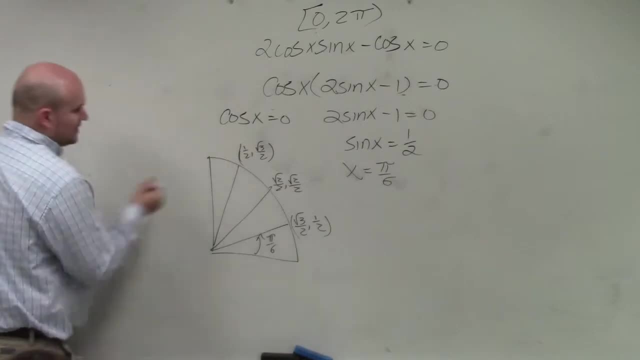 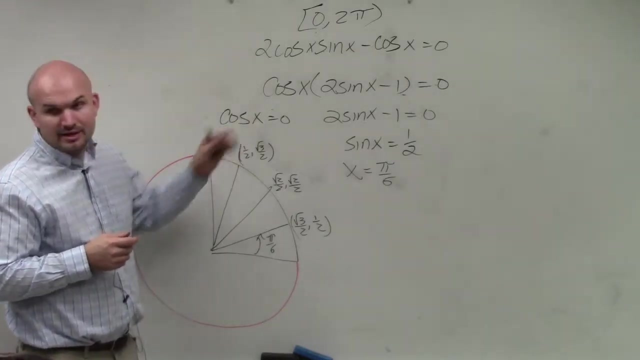 Well, if you guys remember, 0 and 2, pi is basically the whole unit circle. Yes, Yeah, I'm not there yet. I'm going to get back to it. So right now I'm just doing the sine of x1.. 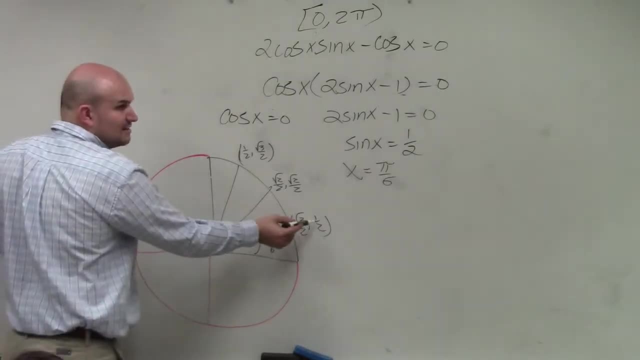 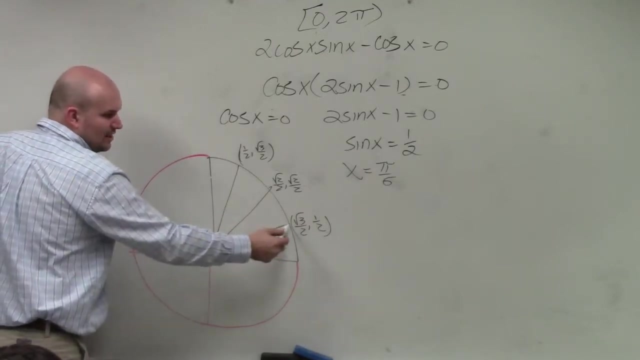 Then, Right, If I look over here, well, here's, Is that a problem? Yeah, Okay, So here's my one angle. right, If I take this angle and I reflect it over here, are the coordinates going to be exactly. 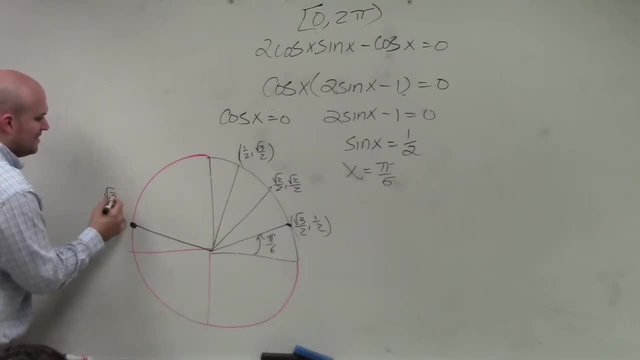 the same. Yes, Yes. Well, they'll be exactly the same, except the x value will be negative. Does everybody agree with me? Does everybody agree with those coordinates? Yes, Yes, is pi over 6,? what do you think? the reference angle of this? 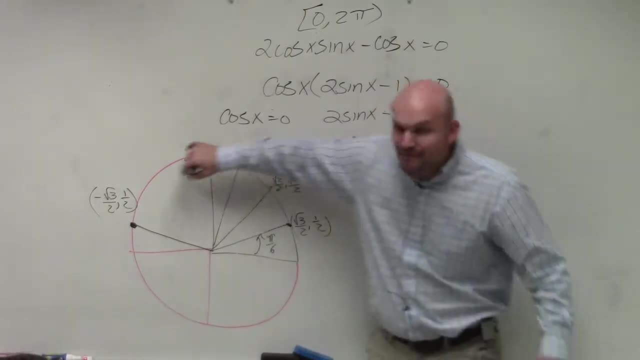 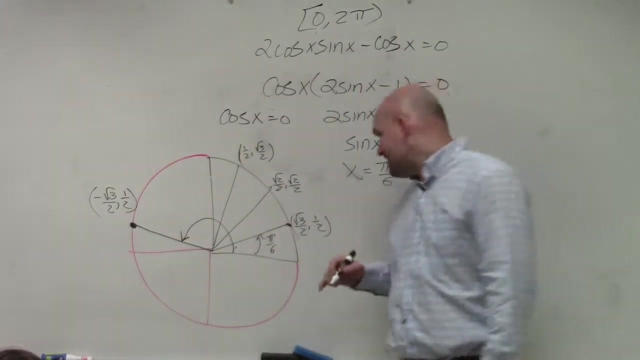 is going to be Pi over 6.. So if halfway around a circle is 6 pi over 6, but I'm short- pi over 6, that means this angle is what? 5 pi over 6.. Good, Got that one knocked out. 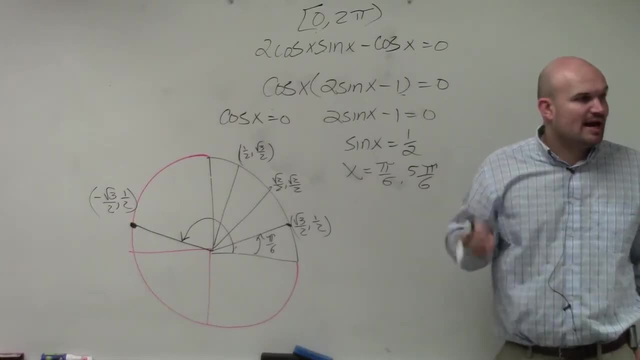 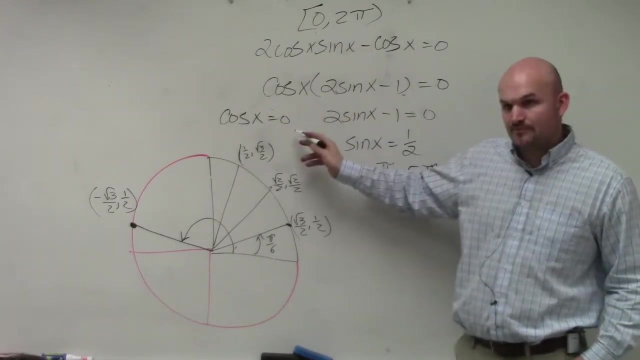 So there's two angles. where sine is equal to 1 half, Does everybody agree with me, Right? Then we've got to find when cosine of x is equal to 0. Well, remember these coordinate points here. this is 0.. 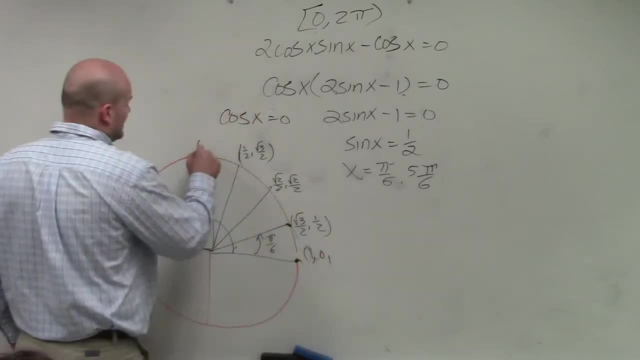 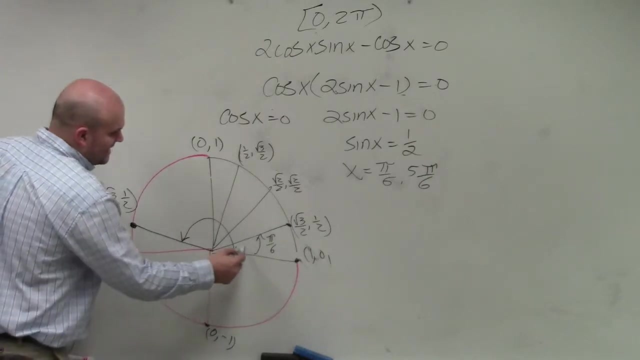 I'm sorry, That's 1 comma 0.. Here 0 comma 1.. Here would be 0 comma negative 1.. Well, hopefully you guys see that this angle here the x-coordinate is 0.. And this angle over here the x-coordinate is 0.. 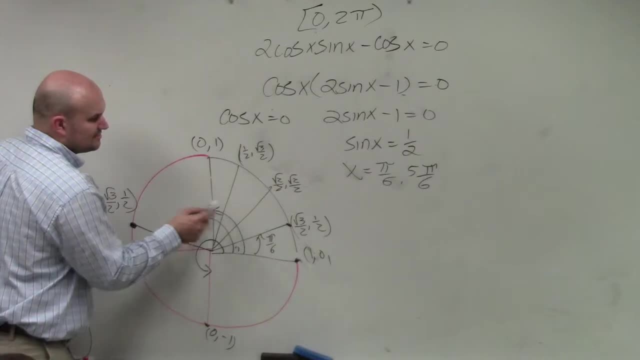 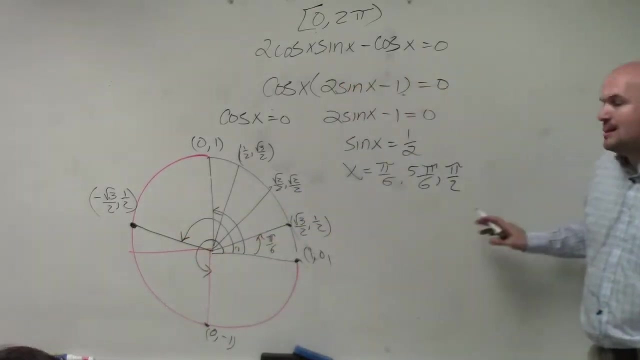 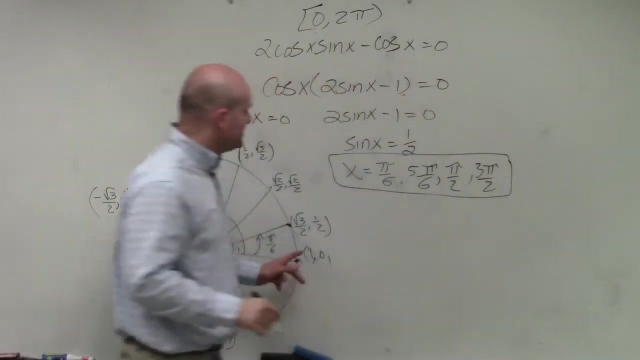 So what is this first angle in terms of Radiance, Pi over 2, pi over 2. Pi halves. And then this angle would be 3 pi halves. So all of the solutions between 0 and 2 pi are right there.